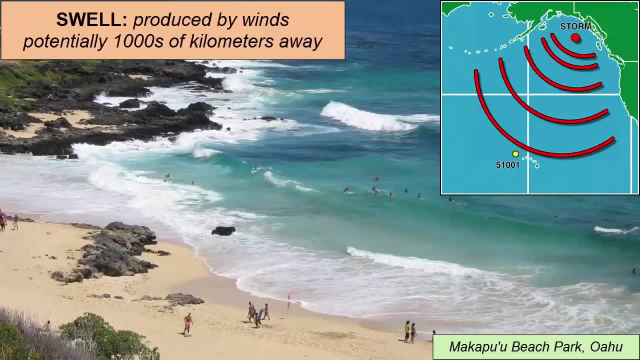 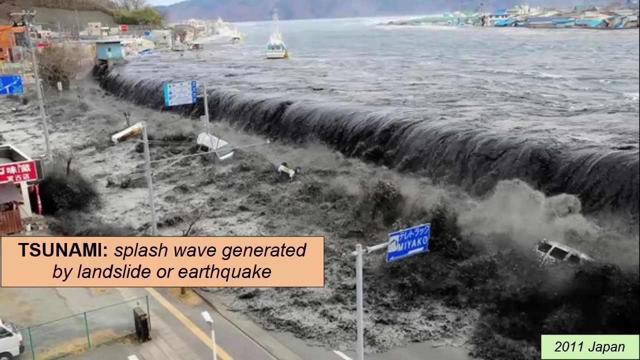 Some waves, called chop or sea, are produced by winds locally, but most of the waves you see at a beach called swell are coming from winds in far distant storms, sometimes thousands of miles away. Tsunami are rare waves that come from a landslide or earthquake that could also have happened thousand miles away. 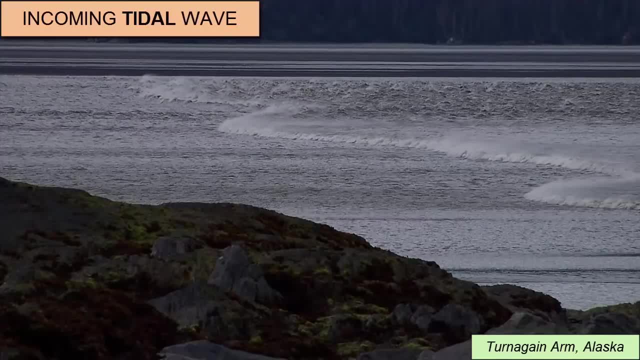 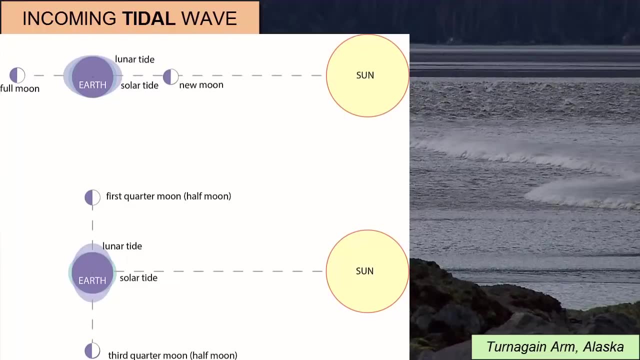 And the most common and consistent waves that hit our beach, usually twice a day, are called tides and are caused by differences in the gravitational forces felt by different parts of the Earth to its neighbor, the Moon, and, to a lesser extent, the Sun. 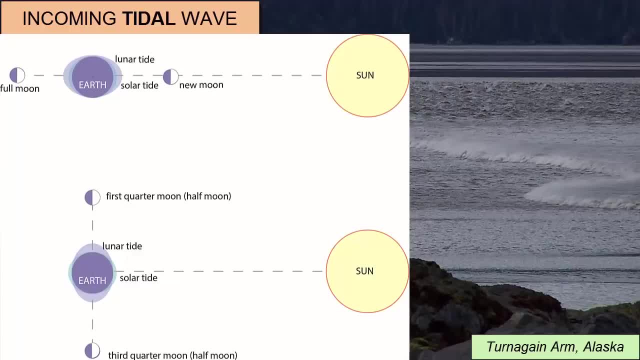 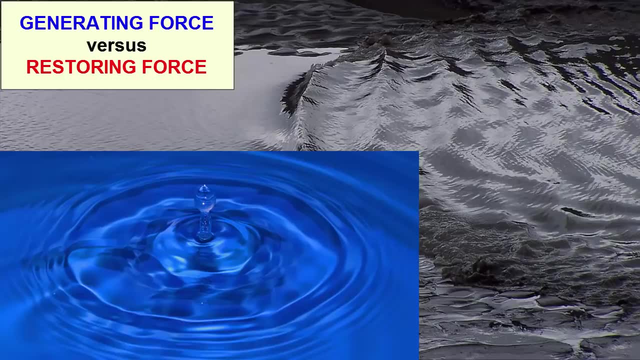 We'll talk more about these tidal waves in a future video tutorial. When discussing wave formation, it is useful to distinguish between the two types of forces that cause waves: the generating force and the restoring force. The generating force is the one that pushes water up across its boundary with the air. 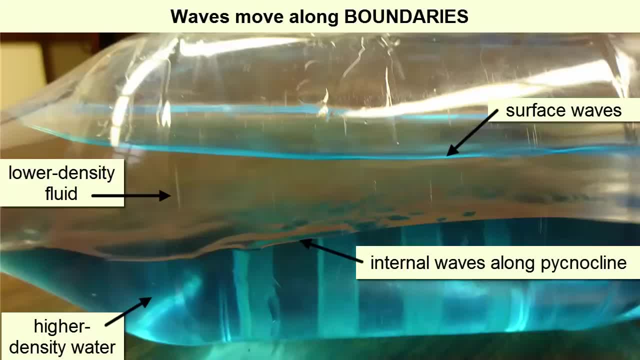 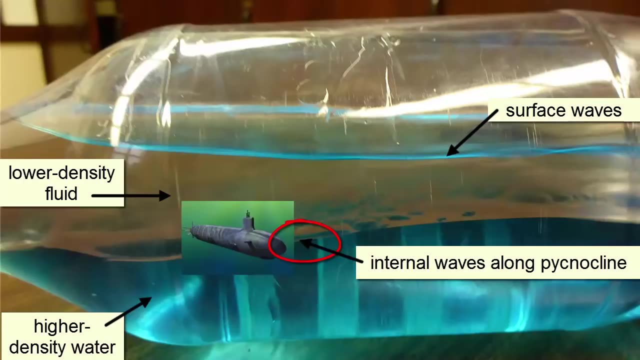 Waves move along the boundaries between two different density mediums In the ocean. we see waves move along the ocean's surface, along pycnoclines within the deeper layers and along the sea floor. Waves that move along the pycnocline can have an impact on submarines and marine life that live along the pycnocline. 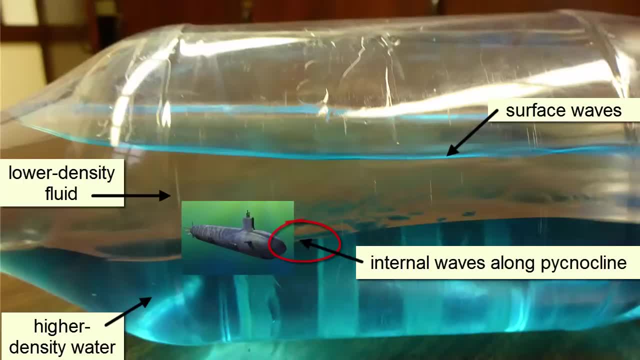 Imagine being in a submarine that is built to withstand only 1,000 meters depth pressures. If it is hanging out in the pycnocline at close to that depth and a wave passes along the pycnocline, the submarine can be moved. 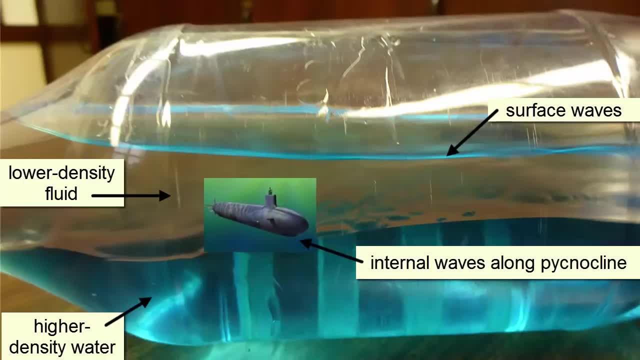 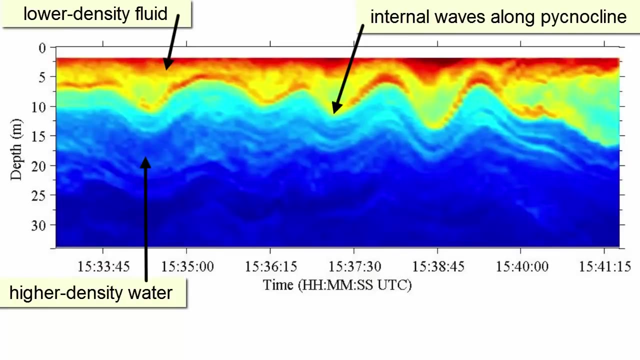 The submarine can be moved by that wave down to deeper depths without warning. It is thought that some of the submarine disasters that occurred without other explanations might have occurred because of this phenomenon. This image shows layers of plankton being moved into a wave shape by waves moving along the pycnocline. 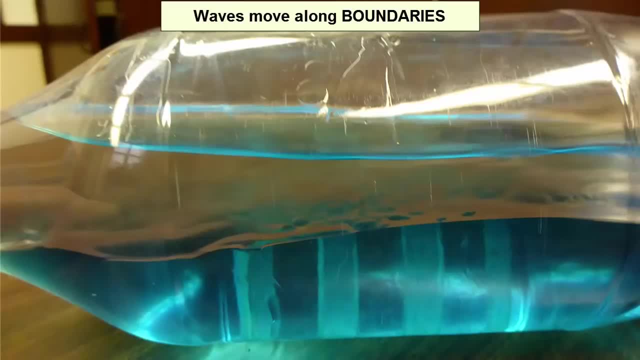 Now that we know where waves occur along boundaries, let's go back to the forces that create them. The generating force pushes water from one layer up into the other layer. The restoring force pulls it back to where it was, trying to restore the balance. 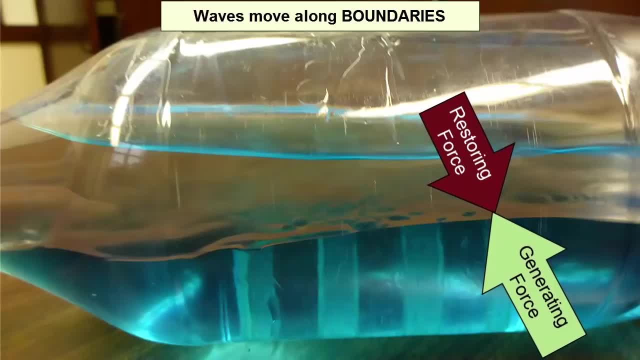 Between the two we get an oscillating motion, And as long as the generating force is continuously pushing and the restoring force continually pulling back, the wave will continue to form in the location of the disturbance and send out its energy in all directions away. 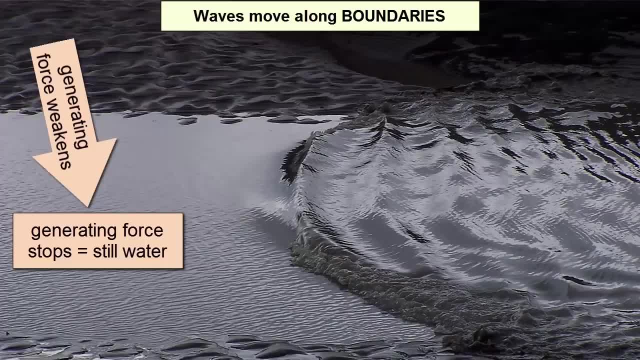 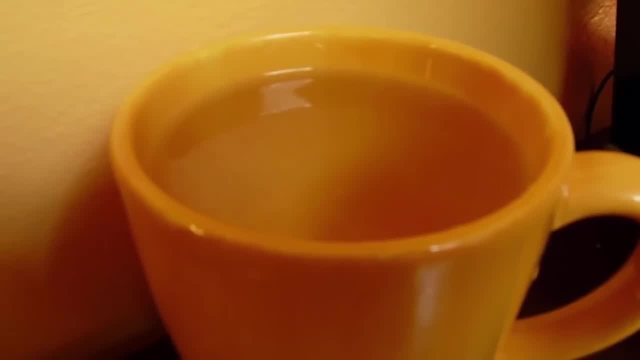 When the generating force stops, the waves all dissipate from the area of the original disturbance and the water returns to its original shape. Let's look at some examples. When you blow on the coffee in your coffee cup, you are creating a small disturbance that is pushing the air boundary into the water boundary. 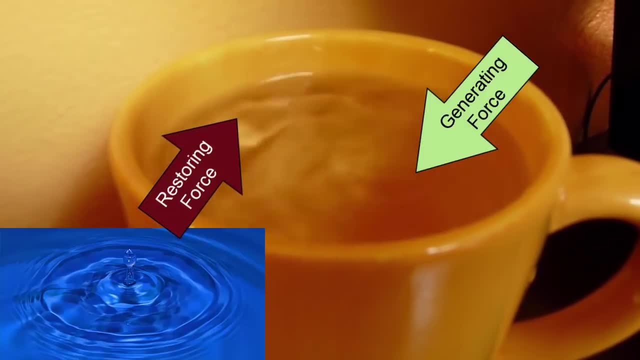 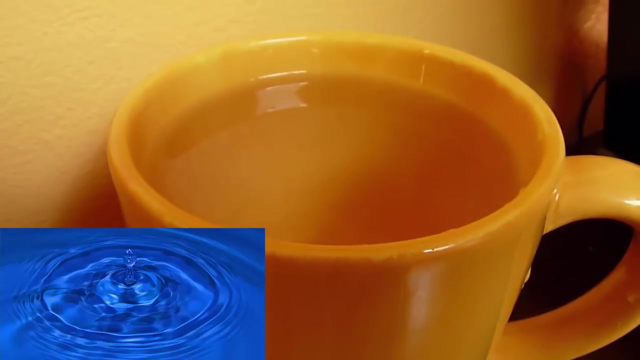 The restoring force in this case is the surface tension of the water which, through hydrogen bonding, connects the water molecules to each other and creates a skin, Small ripples form that emanate out from the area over which you blew. When you stop blowing, the ripples diminish in size and then eventually disappear. 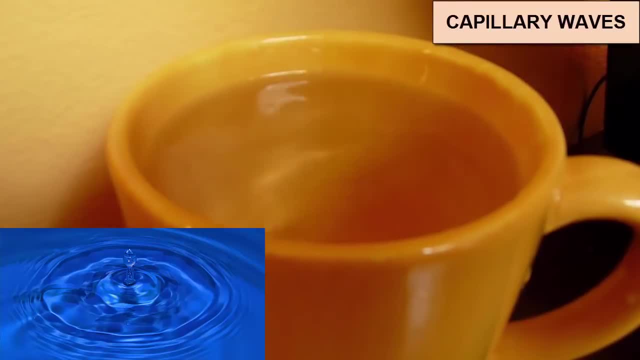 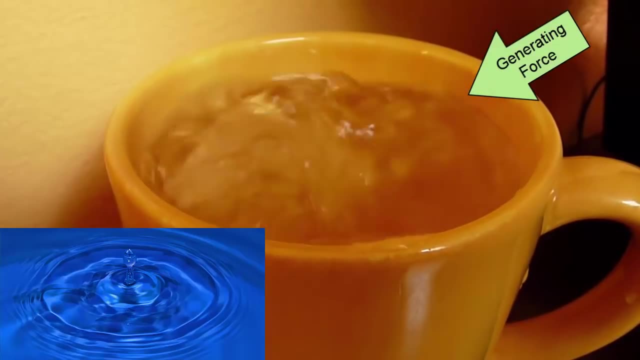 We call these small waves that are restored by surface tension of water capillary waves. If you blow too hard, you will blow the water up into the air, breaking the hydrogen bonds, and the restoring force will now be gravity that returns the water to its original shape. 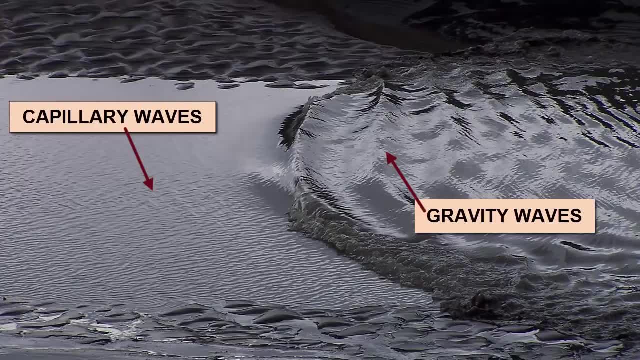 We call waves that are restored to their original shape by gravity gravity waves. When waves are really small, the strength of the hydrogen bonds is stronger than the force of gravity. All waves in the ocean are either capillary or gravity waves, depending upon which is their restoring force. 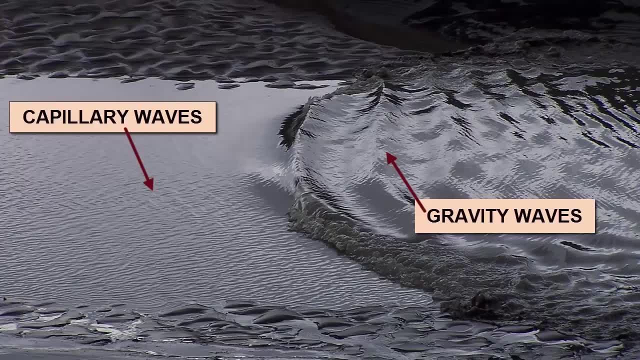 As you can see in this image, if we let wind be our generating force, the main visual difference between the two is their size. The barest breeze will create small capillary waves and as the wind increases in its intensity it will turn into a gravity wave that can get bigger and bigger depending on the force of the wind. 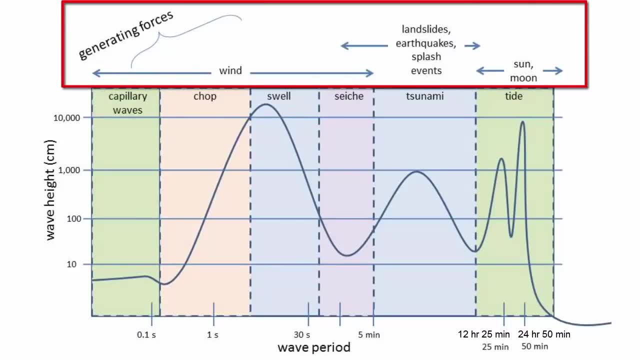 Now let's return to generating force. There are three primary generating forces for waves in the ocean: Wind, displacement of large volumes of water. think of a large splash when you jump in the ocean or when you drop a rock in a puddle. 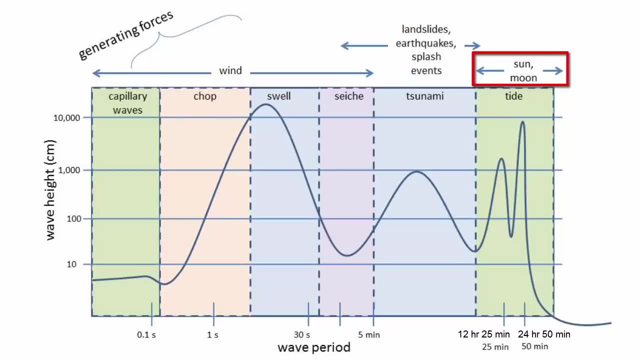 and uneven forces of gravitational attraction between the Earth and the Moon and the Sun. This image here shows these different generating forces and the different heights, periods and names of the waves that are produced. Wind-generated waves include the tiny capillary waves: chop, swell and sesh. 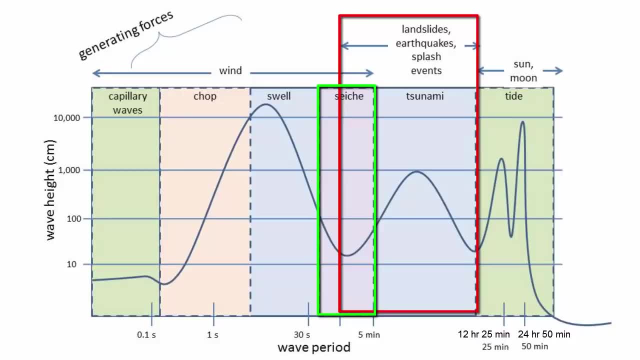 Some sesh can also form through splashes generated by earthquakes or landslides, but most of those waves are called tsunami. As you see from this image, the potential for the tallest waves, as high as 100 meters, occur for swell. 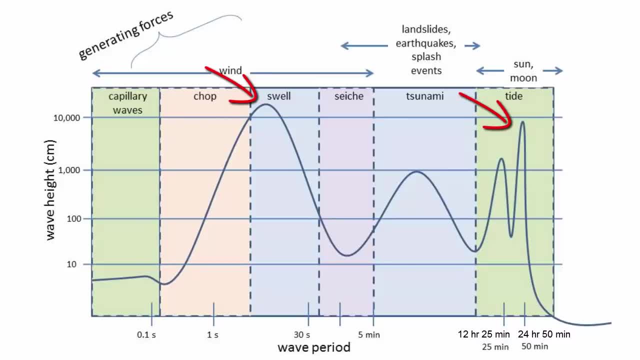 The next highest are tides and the longest period- the longest we have to wait after one wave has hit the shore until the next one comes- is 12 hours and 25 minutes, or 24 hours and 50 minutes, which are the periods of tidal waves. 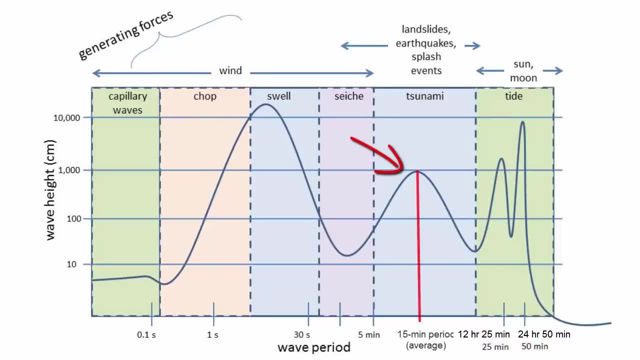 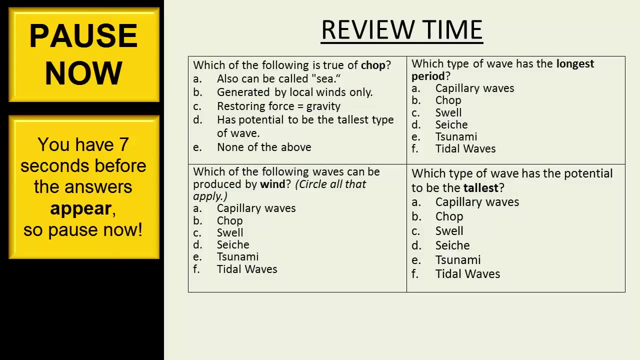 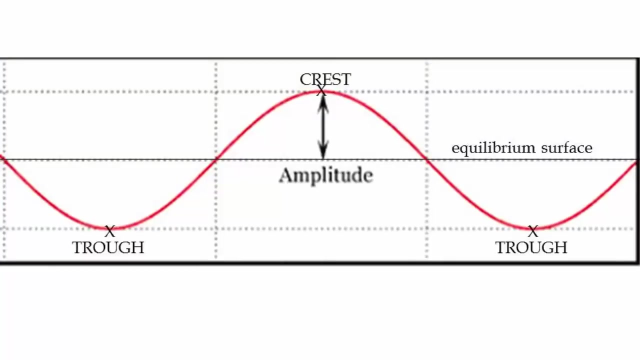 Tsunami, with an average period of 15 minutes, is the next longest. Most waves tend to have periods of a few seconds Pause. now Here is a picture of a fictionalized, idealized wave. The amplitude of this wave is the vertical distance from its midline. 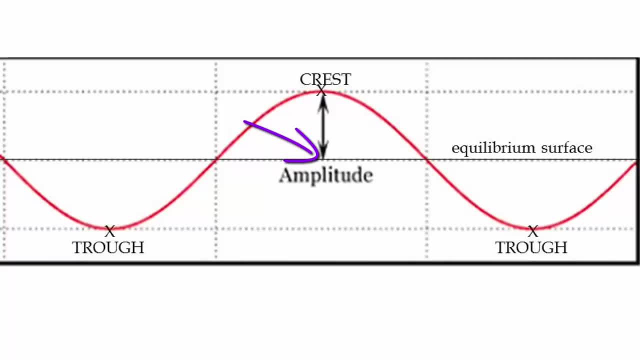 or equilibrium surface, or still water level to its highest point, called its crest. That number should be identical to the vertical distance from the equilibrium surface to the lowest point, called the trough. The equilibrium surface is the level the ocean surface would be at if there were no waves at all. 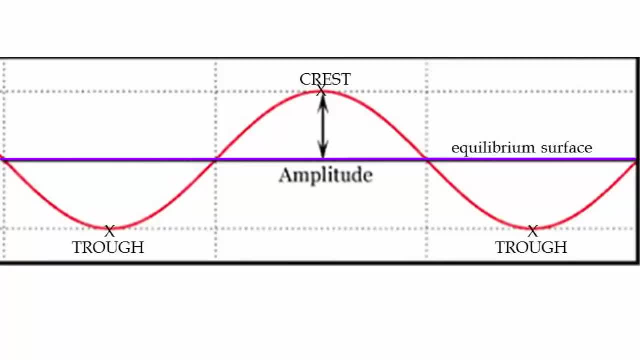 The wave, remember, is a disturbance above and below this line. The height of the wave is the vertical distance from crest to trough. It is twice the amplitude. The wavelength is the horizontal distance from one trough to the next or one crest to the next. 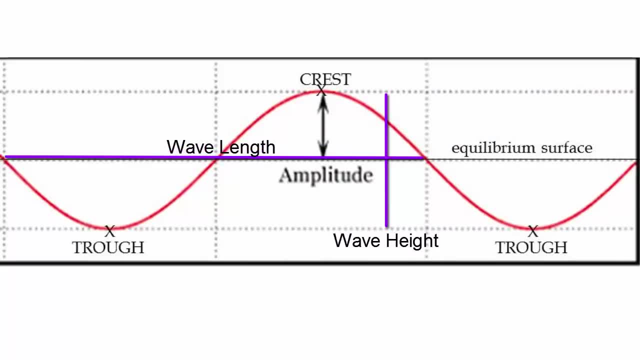 or any one spot on the wave to the place where that exact identical spot appears. again, Based on the definition of wavelength, can you determine how many wavelengths are visible in this picture? Pause now. If you guessed one and a half, you are correct. 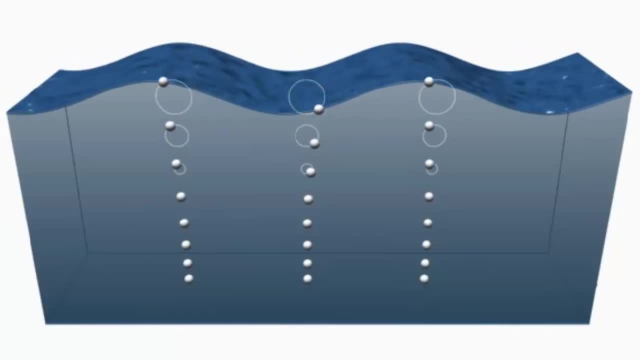 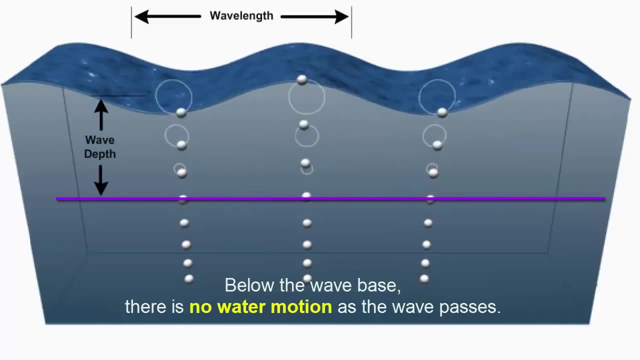 Wave base is another very important characteristic of a wave. It is a depth below the wave under which the water and anything in the water, including fish, scuba divers or submarines, feels no motion, feels no disturbance, doesn't even notice there is a wave above it. 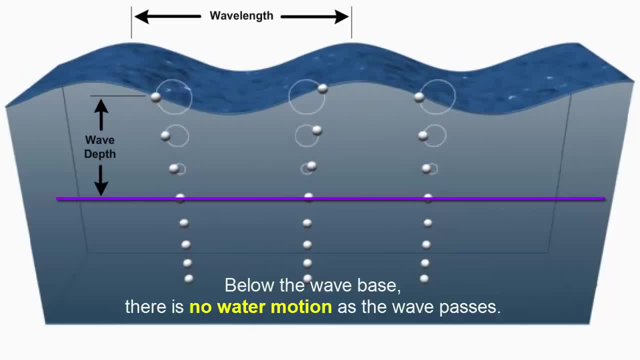 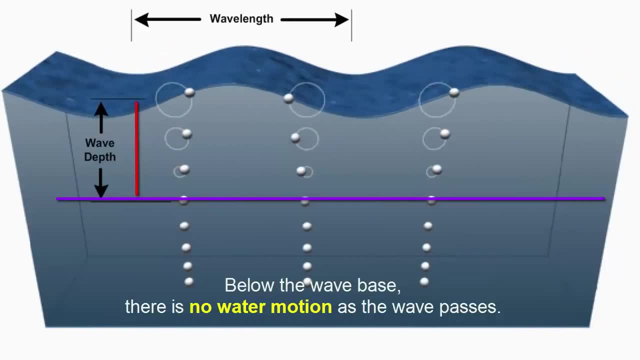 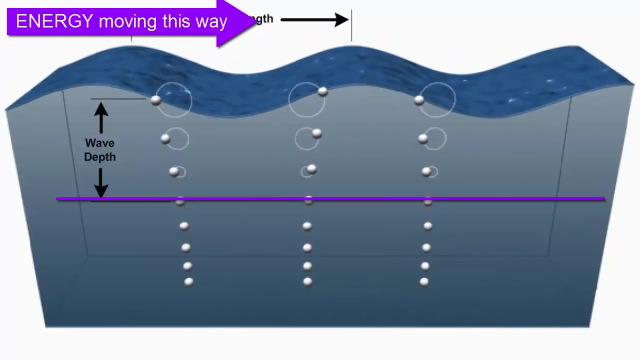 The wave base is calculated by halving the wavelength and then descending that distance from the equilibrium surface or still water level. This image shows what the motion of water looks like as we descend towards the wave base, As waves of energy move across the surface of the ocean. 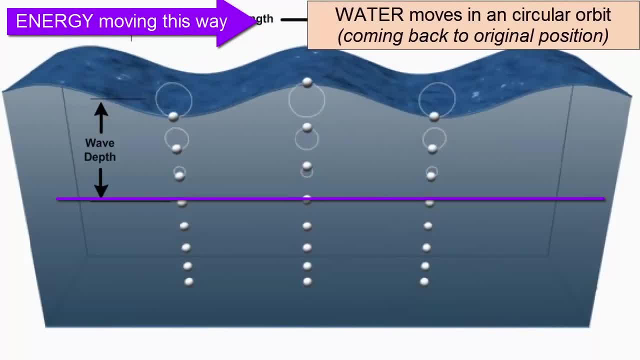 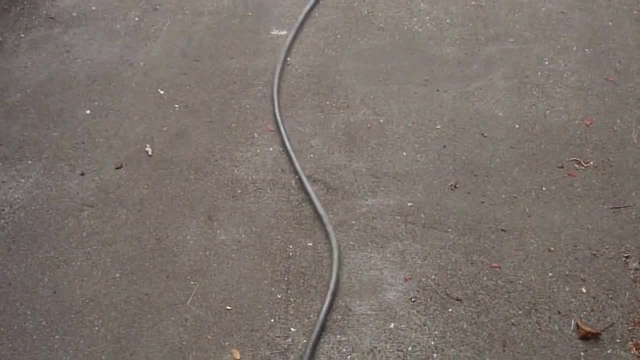 the particles move in a circular orbit, returning to their original position. Waves represent moving energy, not moving water. This video of a slinky will help explain. Although the slinky waves are not the same as ocean waves, they can help illustrate our point. 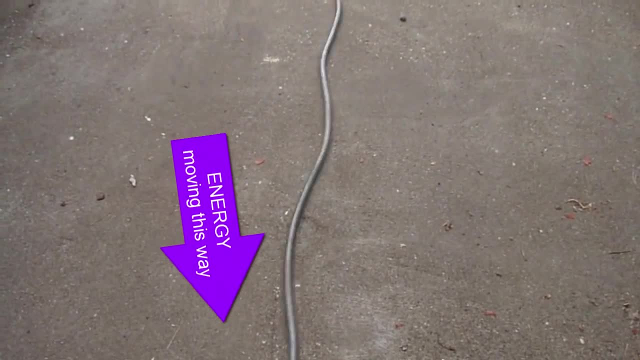 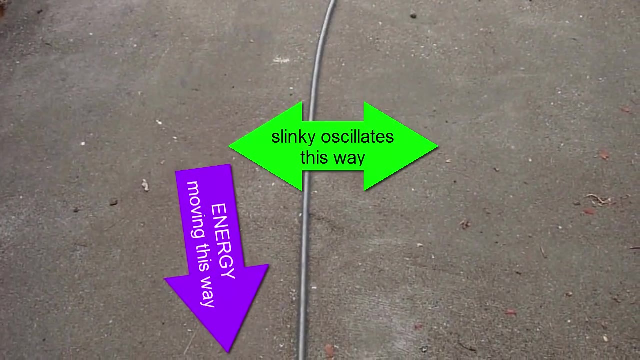 As energy is transferred to one end of the slinky, it makes each individual slinky piece move sideways, returning to its original position. The slinky is not traveling up this concrete driveway, but the waves are. They are traveling up and then back down. 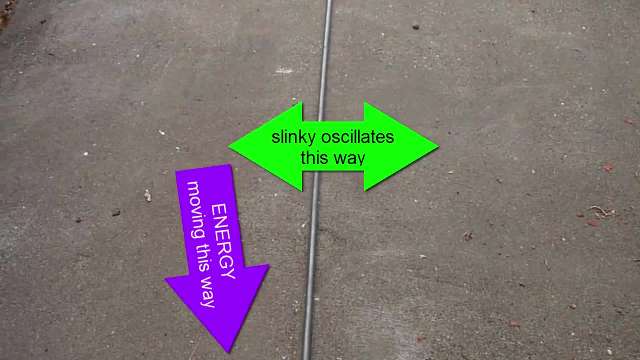 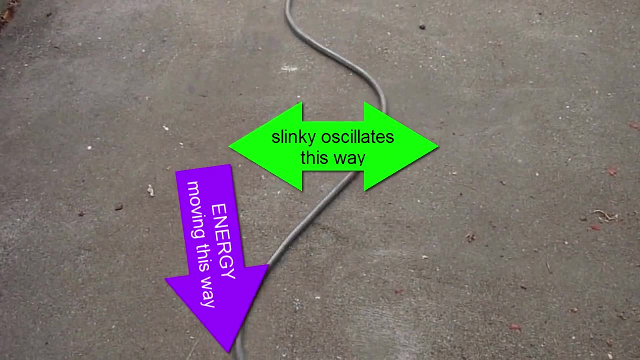 As long as the generating force is continual, the waves will continue moving back and forth. In fact, because the waves are confined to a limited space, they create a standing wave In the oceans. we call these standing waves seches, and they can typically be found in small basins. 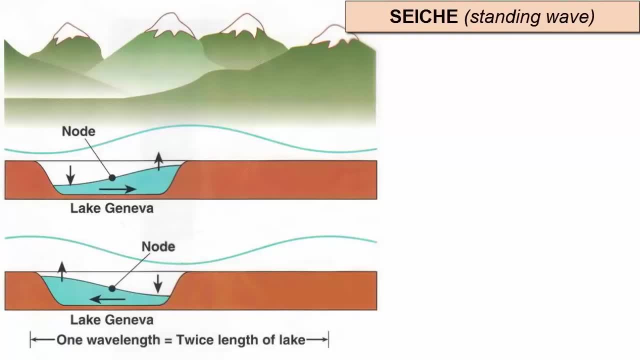 embayments or lagoons. This image from Lake Geneva in Switzerland shows a seche that is a regular feature here due to local wind patterns. The results of these seches are very similar to the results produced by young kids creating standing waves in bathtubs. 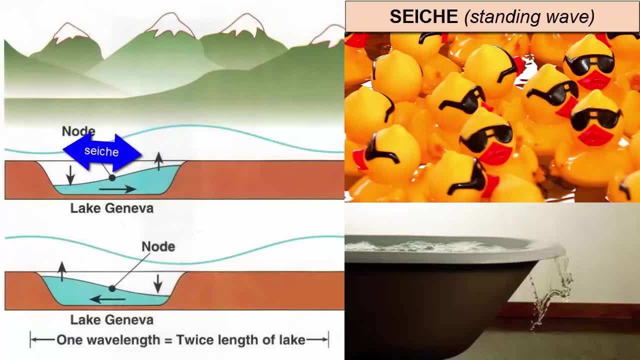 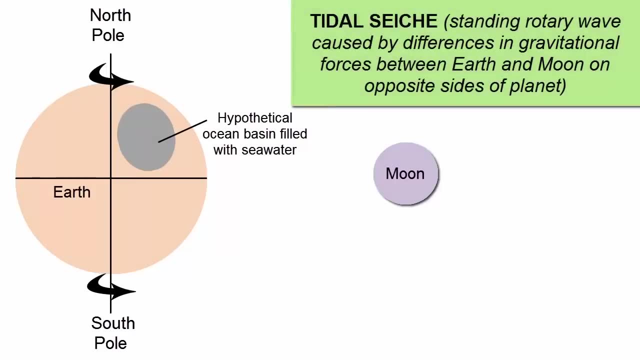 Water sloshes up and over the basin and floods the surrounding areas. The largest standing wave in the world's oceans are the tidal waves. as their generating force, the difference in gravitational forces experienced on different parts of the Earth, for the Moon and the Sun. 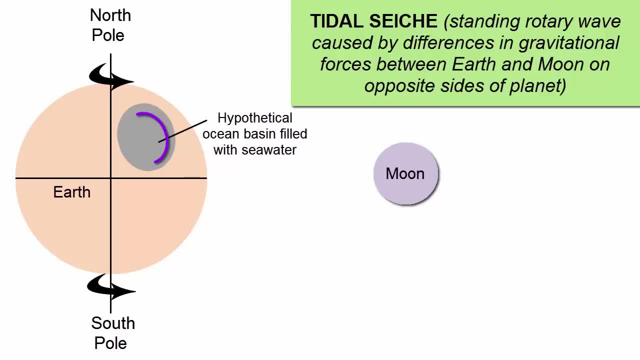 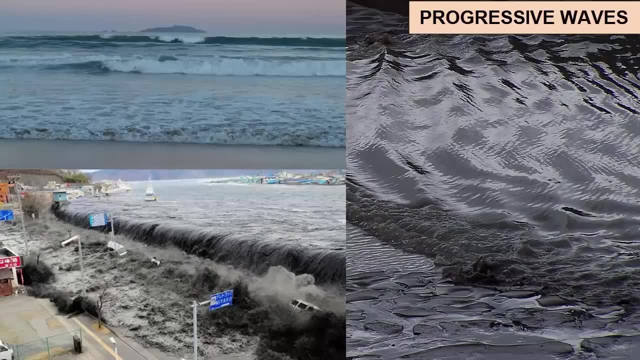 never ceases and they are confined to large ocean basins. In reality, they are simply seches of water sloshing back and forth across the world's oceans. Both tsunami and wind-generated waves in the open ocean are progressive waves. They are generated in one location. 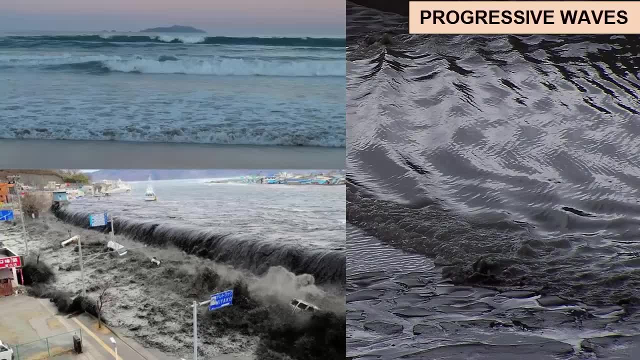 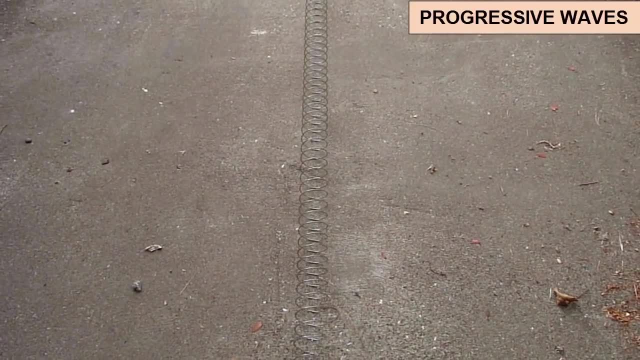 and then move outward from that location, eventually dissipating their energy on distant shores. Their generating force is not continuous. This footage from the slinky shows a progressive wave that dissipates over time. There are two kinds of waves that a slinky can demonstrate. 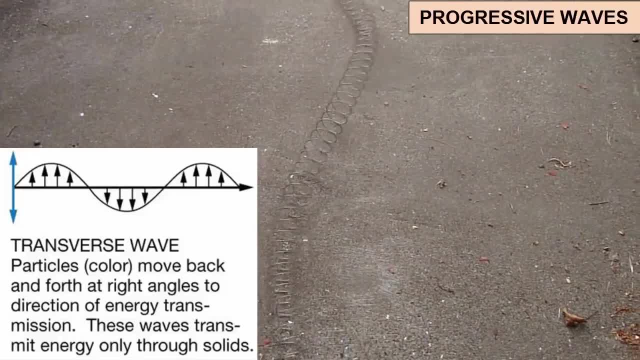 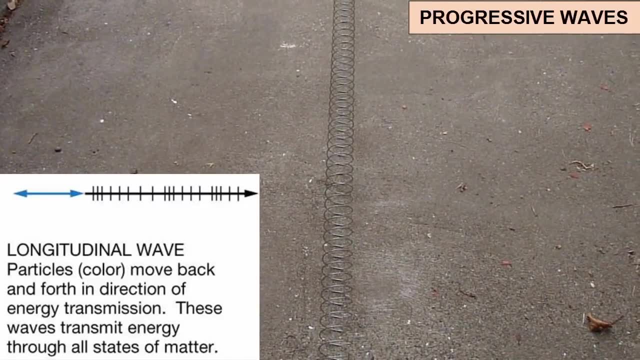 A sideways or transverse wave, similar to earthquake waves that run along the land surface or the bottom of the ocean after an earthquake, and compressional waves or longitudinal waves, another kind of earthquake wave and the kind of wave that sound is. 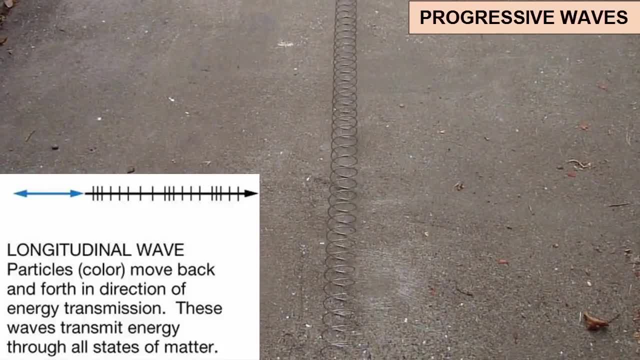 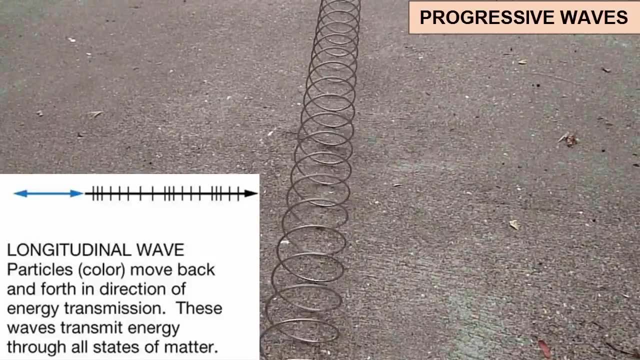 compressing and expanding air as the waves travel from the source of the sound to your ear. Again, in all cases, the waves represent an oscillating motion of the air or water in response to the moving energy. The air doesn't move from the computer speakers. 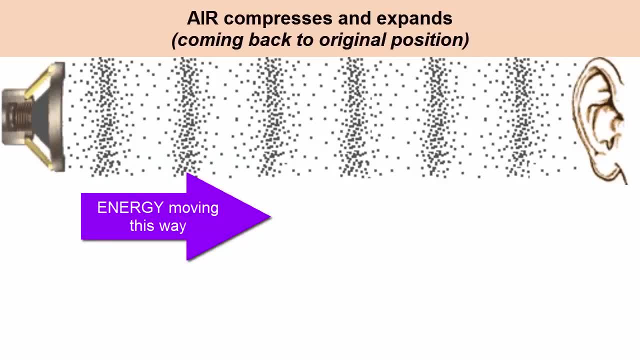 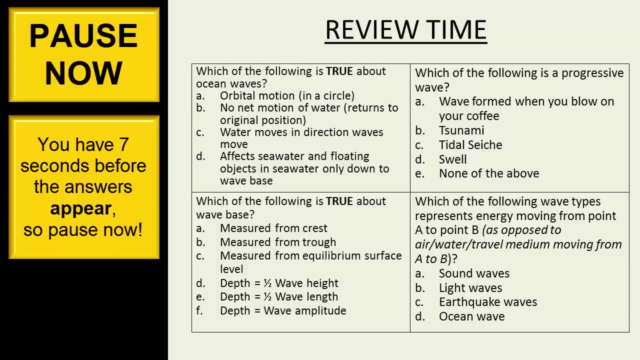 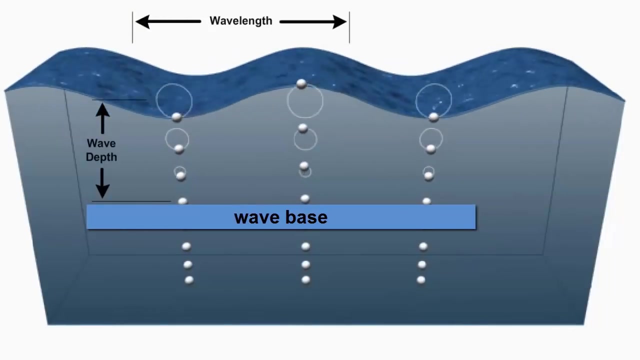 or headphones to your ear. The sound wave moves, The air stays where it is and oscillates as the energy travels through it. Pause now For ocean waves. the oscillation is orbital in a circle, and that orbit becomes smaller and smaller. 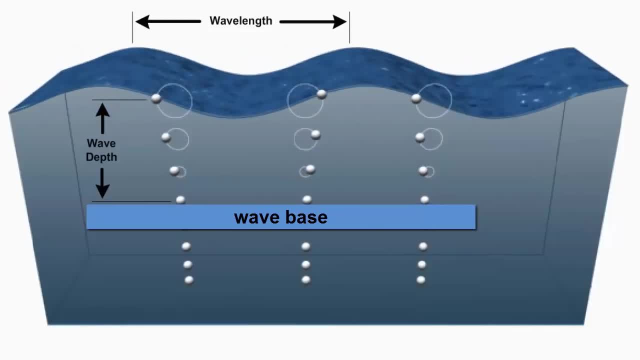 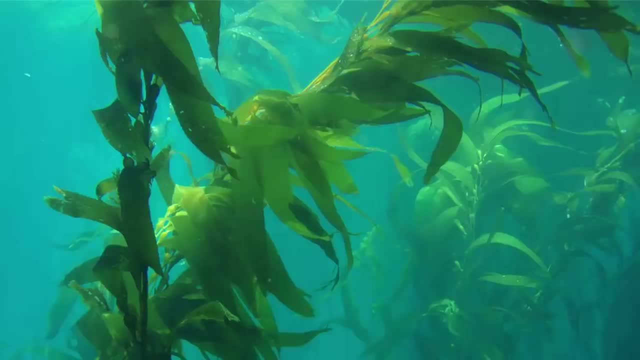 as we descend toward the wave base, below which the oscillation is barely detectable. Everything that is in the water will move in this circular orbit, including seaweed that sits above the wave base, floating garbage or ships or rubber duckies and surfers. 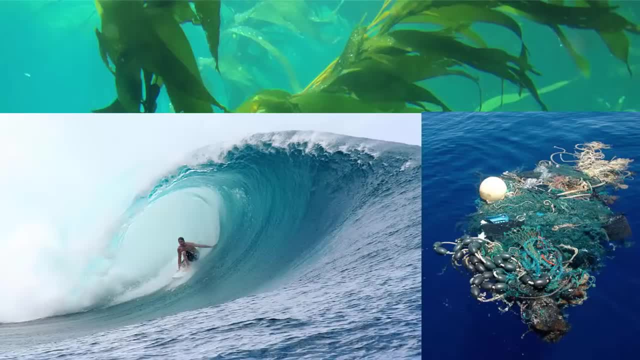 In fact, this perfect curling wave that the surfer has caught displays clearly the orbital motion of waves. In this case, the surfer is heading into the barrel of the wave and is experiencing wave energy in the most hands-on way possible. The period of a wave is how many seconds? 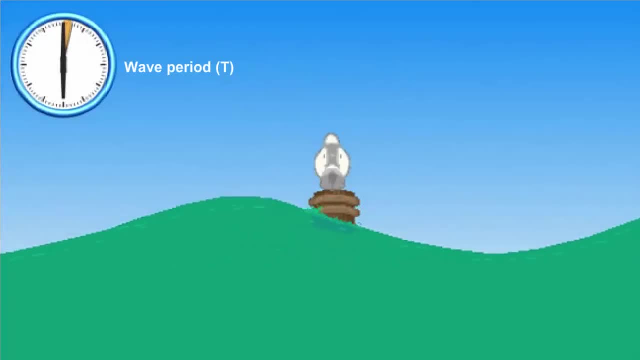 minutes or hours pass between waves. Imagine being on the beach and hearing a crashing wave. Count the seconds until the next wave crashes, and that's the period. Of course, that's assuming that the waves that are crashing on the beach are all part. 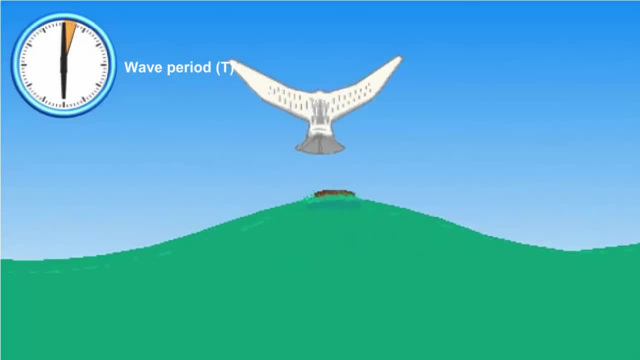 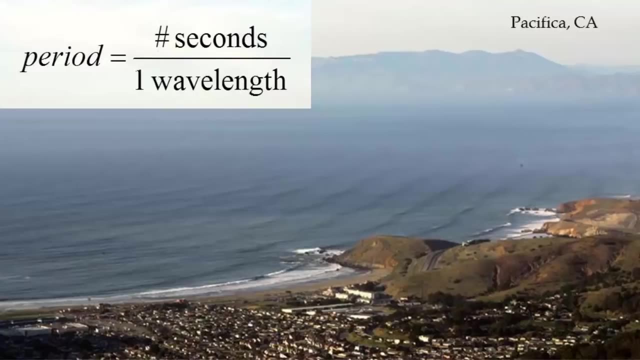 of the same set of waves. In fact, there are often many different waves from many different locations approaching the beach on any given day. at the same time, However, in this picture of Pacifica, California, we can see a regular set of waves called swell. 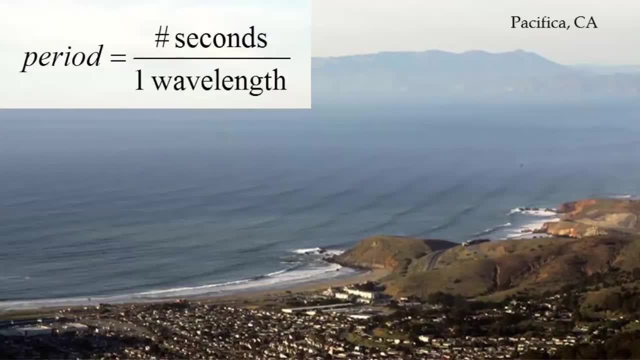 that seem to be coming from one direction. The period of these waves is probably around 10 seconds. That means every 10 seconds you can hear a wave crash on the beach. or if you wait one minute, you should expect to experience six waves. 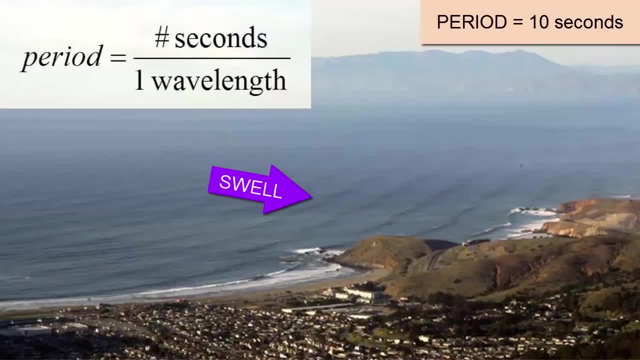 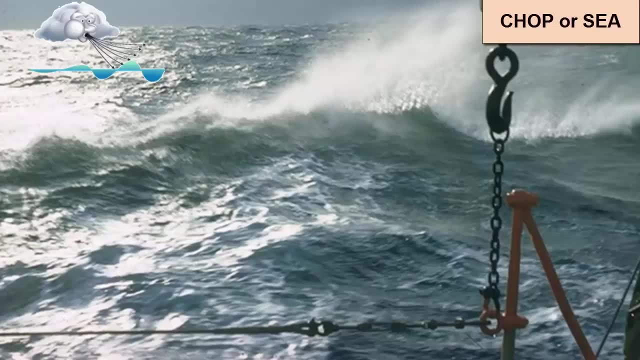 Where are these waves coming from? There's no local wind producing them. However, thousands of miles away, there is a storm system, perhaps a hurricane, perhaps a winter storm, And the waves that are kicked up in that area are called chop or sea. 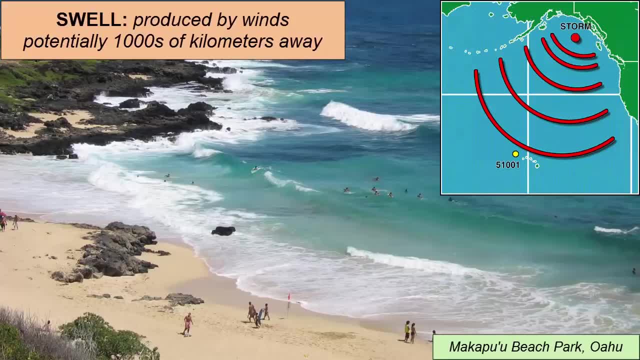 When they propagate outward from that storm area, they separate into regular sets of wave trains, all waves within which have the same height, wavelength and period. These ordered groups, or sets, are called swell, and they travel thousands of miles to our beaches. 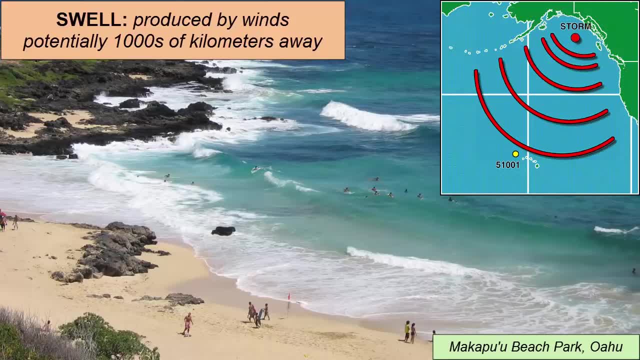 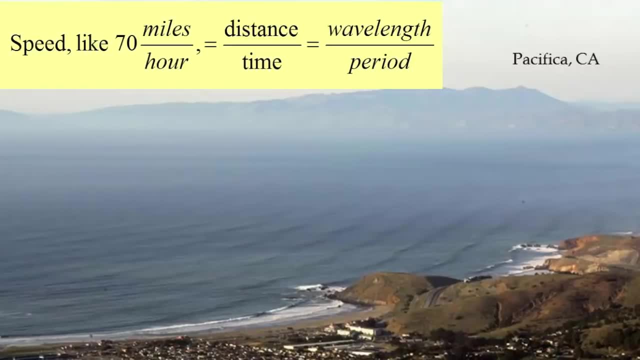 What happens to them when they arrive? To answer that, we have to review a few more concepts. Let's talk first about wave speed. Like the more commonly known, speed we associate with our cars on the highway, speed is simply distance over time. 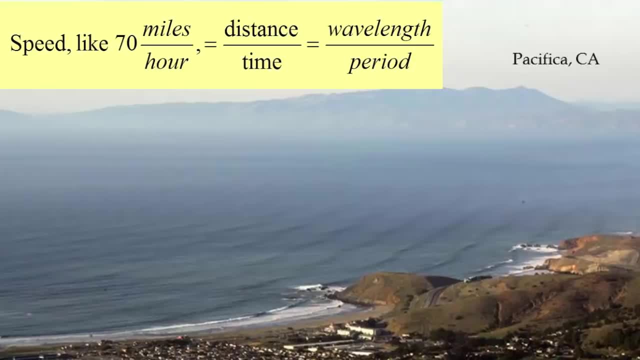 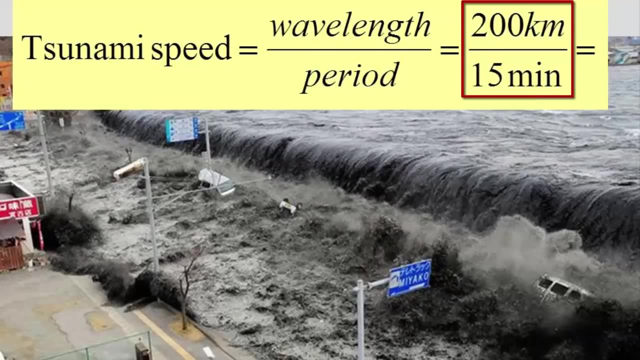 For a wave, the distance it travels in a given unit of time is its wavelength over its period. For example, tsunami have an average wavelength of 200 kilometers and an average period of 15 minutes. When we divide those numbers, we get an average speed of a tsunami. 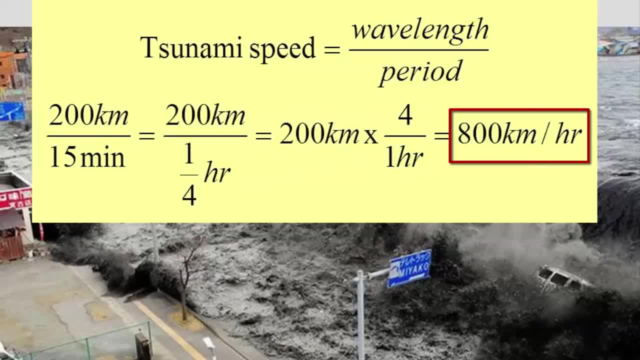 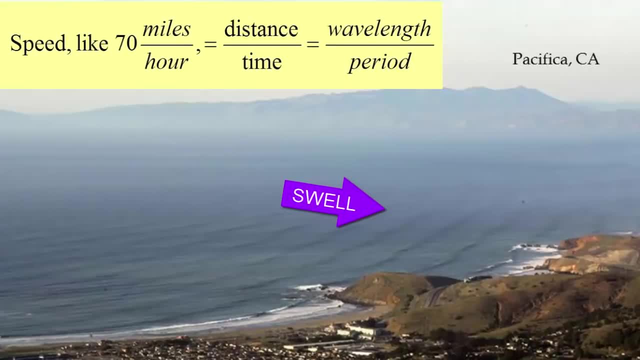 of 800 kilometers per hour. That's how fast the average speed or energy of a tsunami wave travels across the ocean. Swell that approach our beach tend to move at speeds more like 33 kilometers per hour. However, that speed will slow once the wave feels bottom. 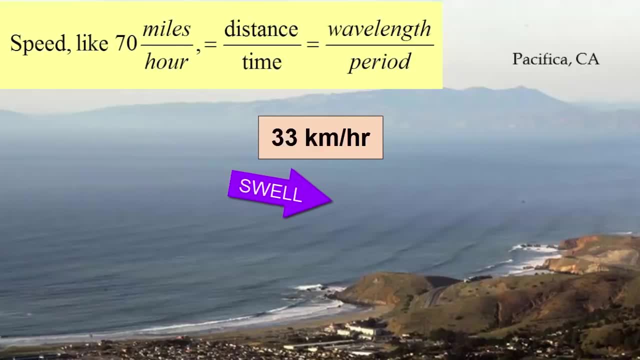 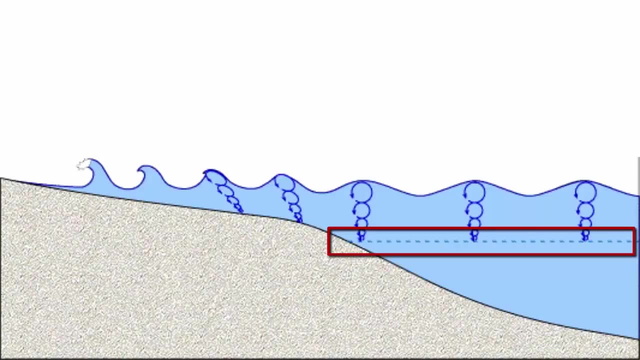 which means once it enters water shallower than its wave base. This image reviews the wave base as the limit of orbital motion below a wave. We call waves that move through water deeper than their wave base deep water waves. Note that this definition has nothing. 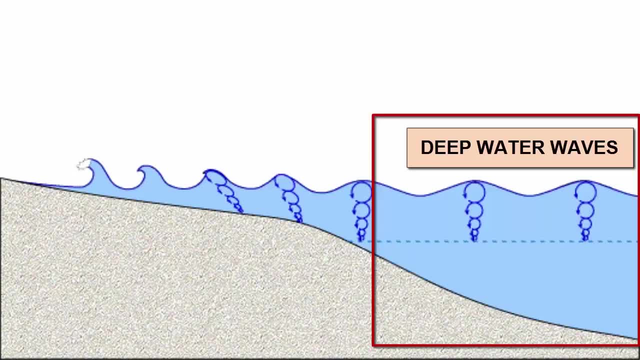 to do with whether we think the water is deep or shallow, but only if the wave does. If the wave's base is above the sea floor, it feels like deep water and there's no interaction between the wave and the sea floor Once a wave enters water that is shallower. 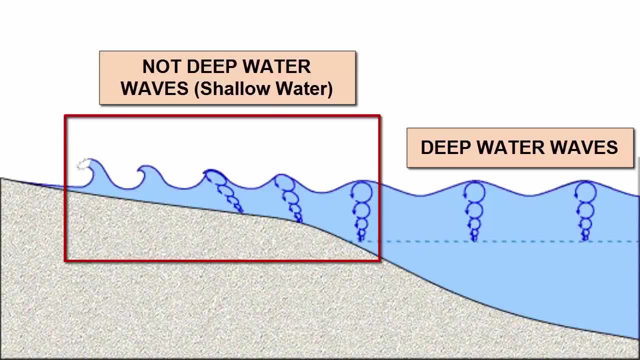 than its wave base. it now transfers its orbital motion to the rock or sediment on the sea floor. That transfer of energy will pick up and move sediment, erode rock and generally cause a frictional slowing of the base of the wave. The top of the wave might still be moving. 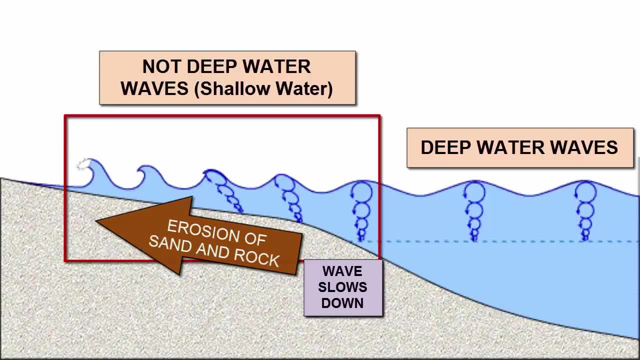 at its original speed, but the base is slowing down. This causes waves to bunch up. their wavelengths decrease, grow taller and have their circular orbits squashed into elliptical orbits. The transformation of a wave as it enters shallow water: slowing and growing taller.